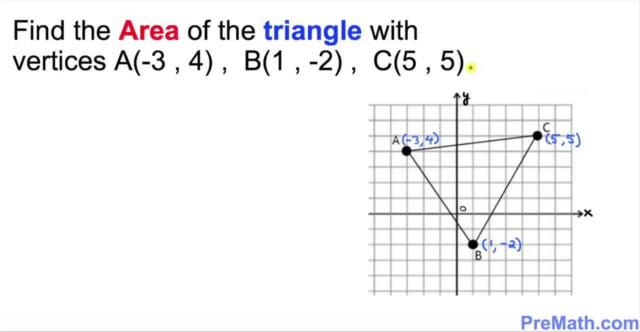 Hello again everyone. In this video tutorial we are going to find the area of the triangle with these three given vertices- Sometimes we call them the points- And over here on the xy plane, you can see all these three coordinates of these three vertices. So the very first thing, I 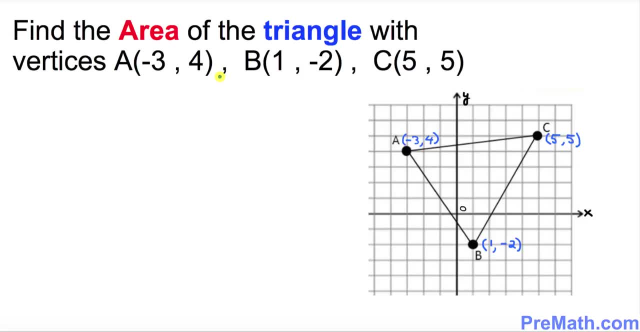 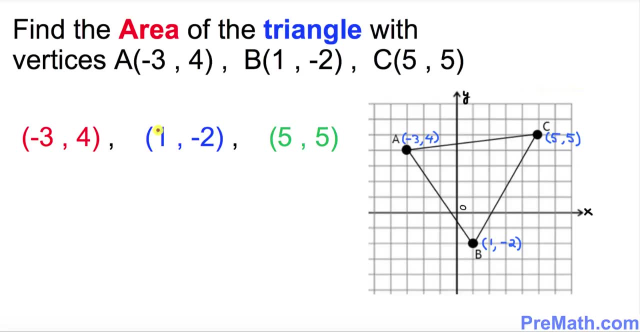 want you to just focus on the coordinates of these three vertices. And here, in the very first step, what I did is I put these vertices, or the coordinates, in different colors. With this one, with the red color, I want to call it x1, y1.. And the second point, I want to call it x2, y2.. 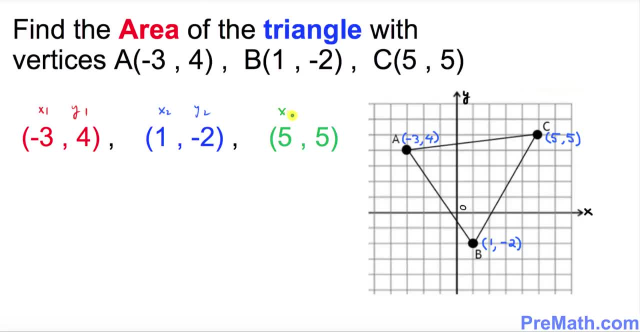 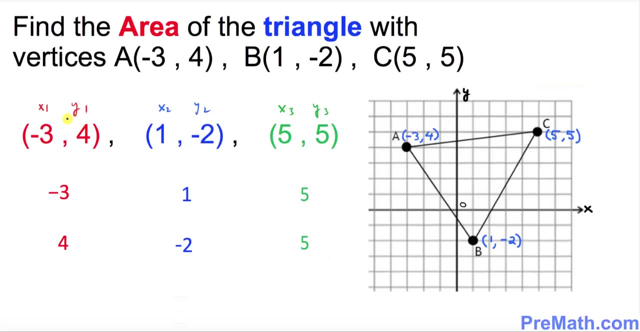 And the third one I want to call x2, y2.. And the fourth one, I want to call it x3, y3.. I use these different colors to make sure that my student will comprehend in a simple way. And in this next step, I want you to convert. 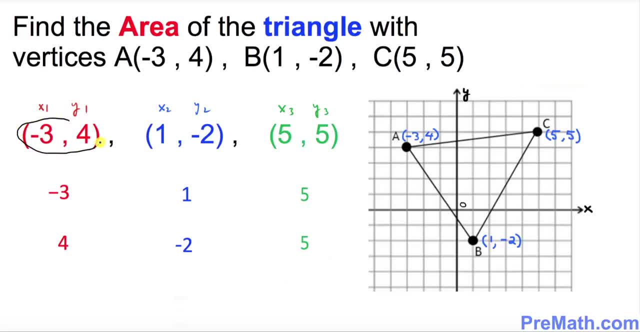 these coordinates from horizontal position to a vertical position. As you can see, these are in horizontal position. I want you to just convert it into horizontal, A vertical position. that's going to make our job a lot easier. From horizontal to vertical. 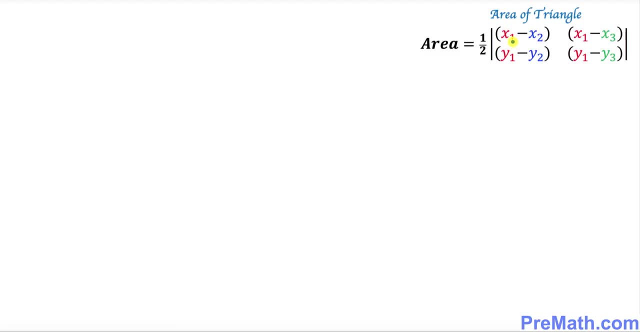 So far, so good. Now we will be using this formula to find the area of a triangle. If you don't understand this formula, don't worry. I'll try to make it really simple that you won't even need this formula. And now, in this next step, we're going to be finding the area. 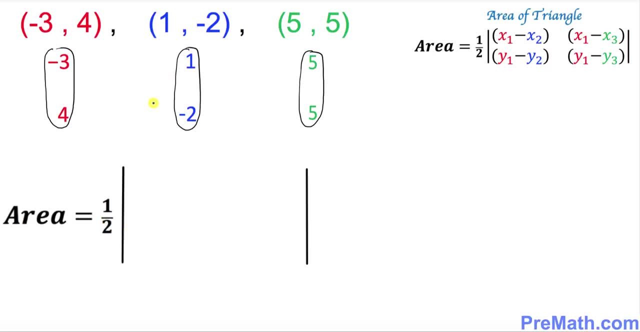 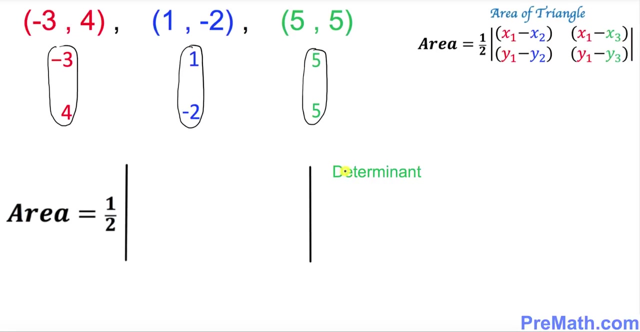 of the triangle by using these coordinates, by filling out this box, By the way, this box, that you can see these vertical lines, this is much like this is related to matrices, And now this is called determinant, as you can see. Now I'll explain more about determinants. 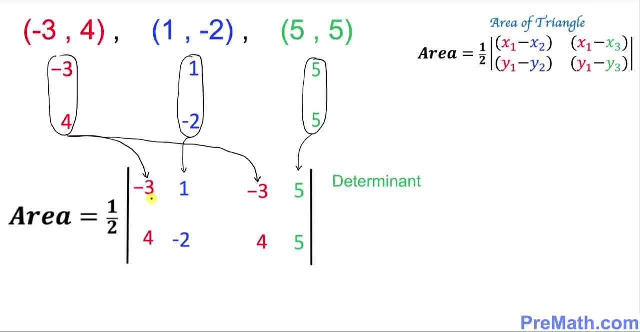 in the next few steps. I have filled out this determinant, this box by just putting these red numbers. You can see, I put red numbers right up here and over here, as you can see, And then blue only in one column and the 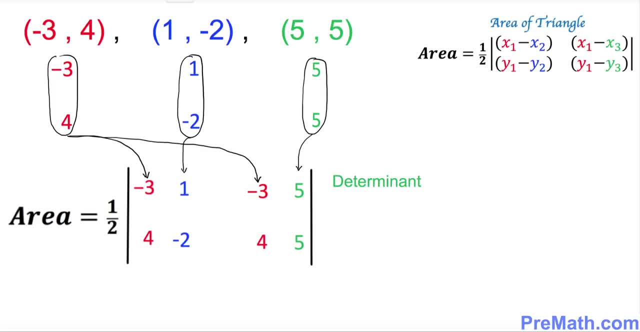 green in one column as well. So the next step is really, really simple. In these two numbers you see negative three and one. I want you to put a minus sign in between them, Always minus sign in between them, And then I'm going to put a minus sign in between them, And then I'm going to put a 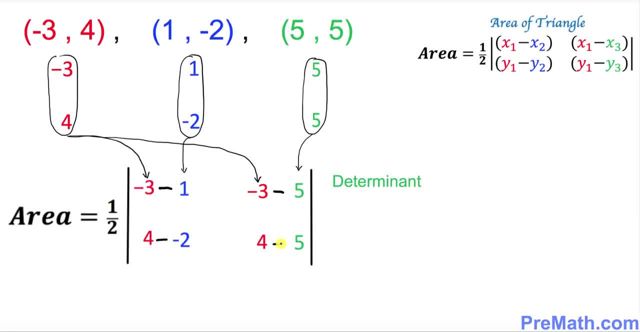 minus sign in between them, Minus sign in between them and minus sign in between them. And now our next step is going to be really simple. Okay, let's go ahead, And this is area is going to be equal to one over two times. Let's simplify this one And what we get? negative, three and negative. 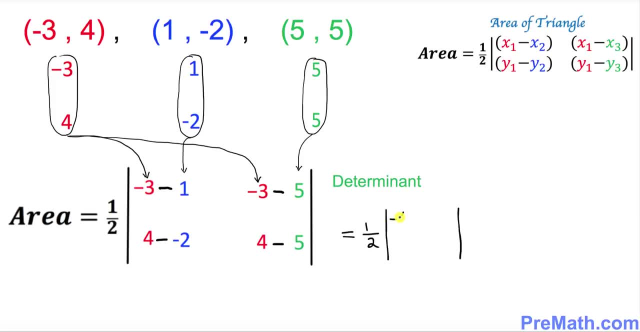 one. If you simplify, that's going to give you negative four, isn't it? And this is going to give you negative eight. This you see whenever you have a negative and negative that gives you positive sign. Four plus two is six, So this makes really simply six, And four minus five is negative. 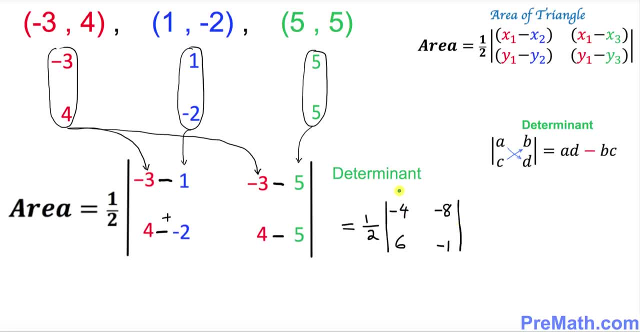 one. And finally, we're going to find the value of this determinant by using this formula which says: if you have A, B, C, D, then you just simply crisscross A times D, and then you put always minus sign and then minus B times C. So this is what I will be doing. 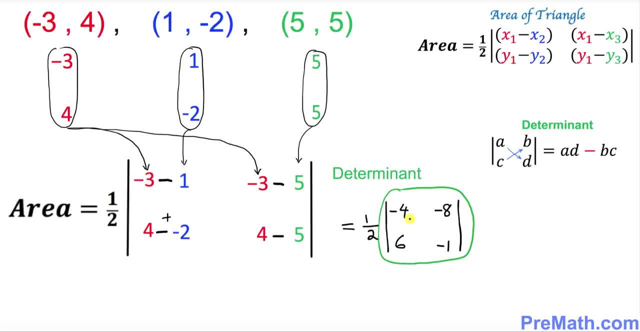 I want you to go ahead and cross multiply this way first, So negative four times negative, one is going to give you four, isn't it? And then you always put a minus sign in between. And then I want you to cross multiply this way first, So negative four times negative one is going to give you.